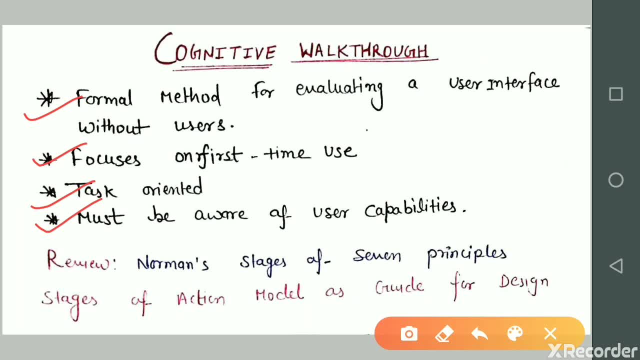 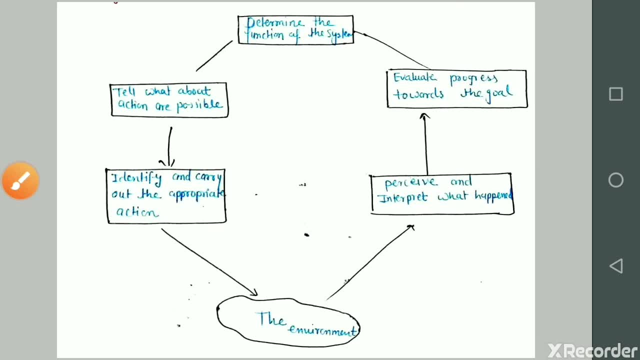 I have discussed in the previous lecture, number 9.. So you can see Stage of actions models as guide for design. This is the model. So first determine the function, Then what action are possible for the particular function And then identify a particular action. 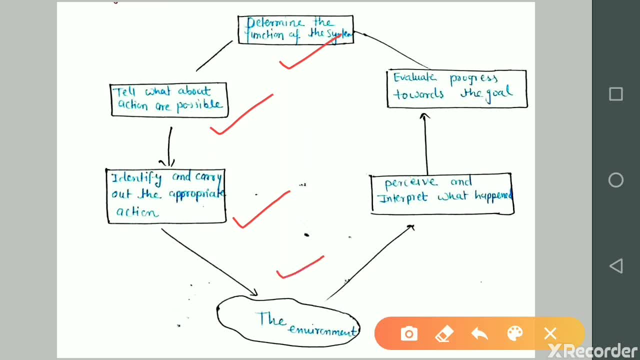 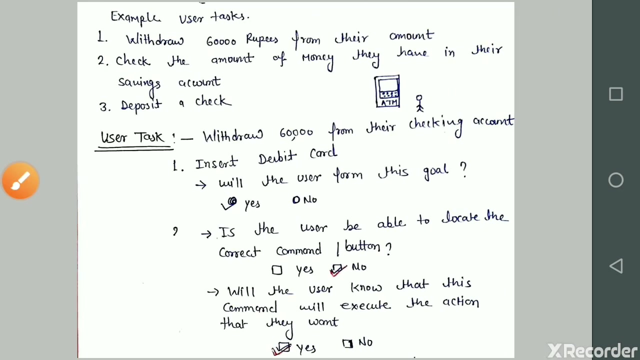 After that, set environment And then perceive the interpret what happen when you create a action. Last is evaluate the progress towards the goal We have already discussed in the normans principle cycle. You can see my lecture number 9.. And then we have example of ATM machine. 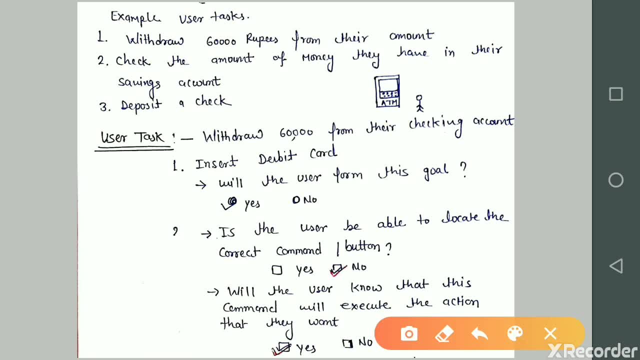 And then we have three tasks to interact a user with the ATM- So this is a ATM And this is a user- And user interact with the machine. And then we have three tasks to interact with the ATM machine. First is withdraw. 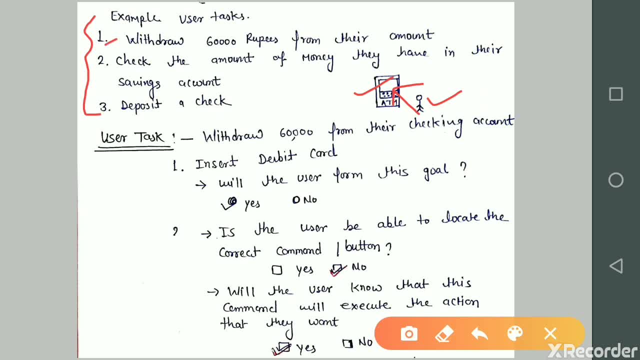 Withdraw 60,000 rupees from their amount And then check the amount of money they have in their saving account, And last one is deposit a cheque. So these are the tasks. After that, first task of user is withdraw money. 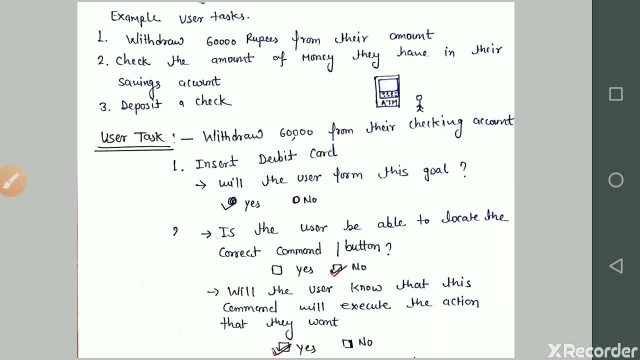 So how we can withdraw money from the ATM machine. So what is the first starting process? Withdraw 60,000 from their checking account. First, insert debit card. So when the user form this goal? if yes, is the user we able to locate the correct command? 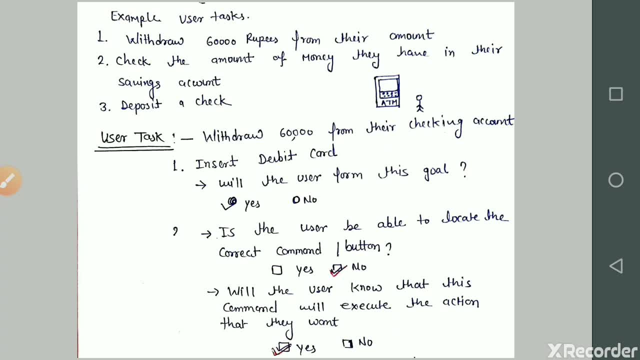 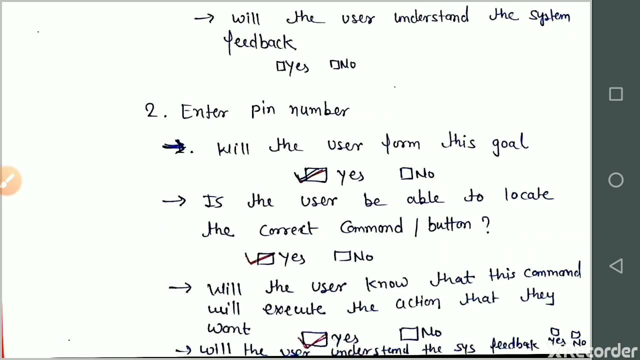 If yes or no, select according to user. And then third question is: will the user know that this command will execute the action that they want? If yes or no, according to user. After that, will the user understand the action? give feedback? yes or no? 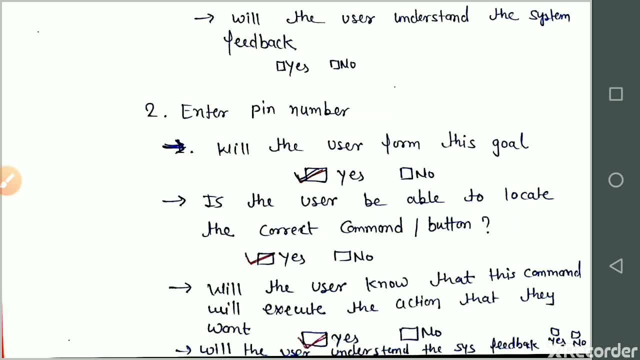 user and second task, according to the user, is enter pin number. will the user form this goal? yes, is the user be able to locate the correct command button? if yes, will the user know that this command will execute the action that they want? if yes, will the user understand the system? 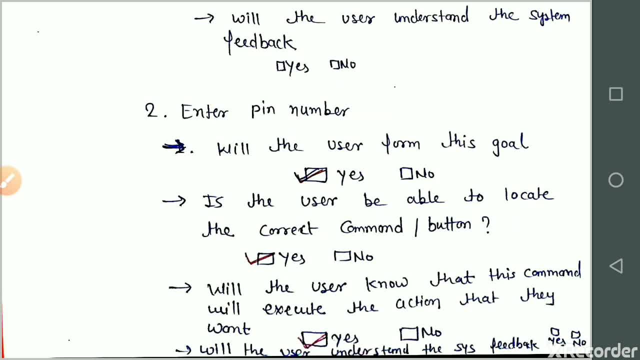 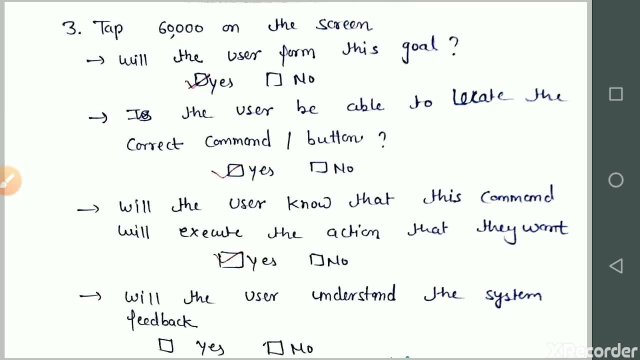 feedback. if yes or no, according to user, user can choose one, yes or no. third task is tape 60,000 rupees on the screen and will the user form this goal? if yes, is the user be able to locate the correct command button and if yes, will the user know that this command will execute the? 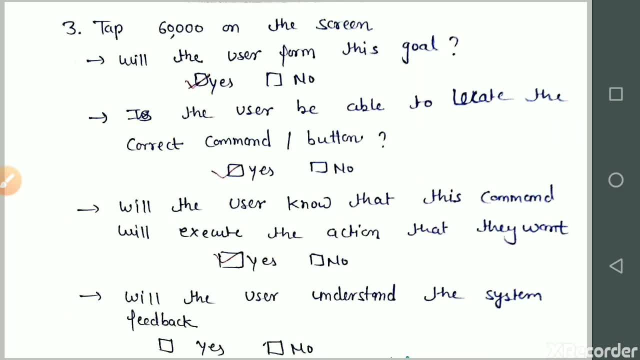 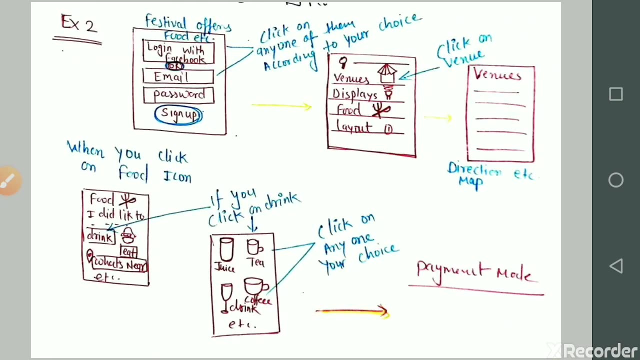 action that they want? if yes, will the user understand the system? system feedback yes or no, they can collect money or they can't be collect the money. these are the tasks now we can take another example of if you are using net and suddenly you saw a addy add on. 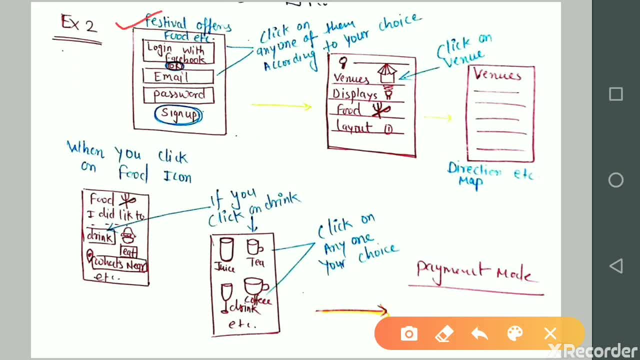 your screen. that is festival offer foods. so, first of all, what you do, click on anyone from them according to the choice- like you can log in with Facebook or you can log in with Gmail- and select anyone from them, and then you can sign up. click on any one of them according. 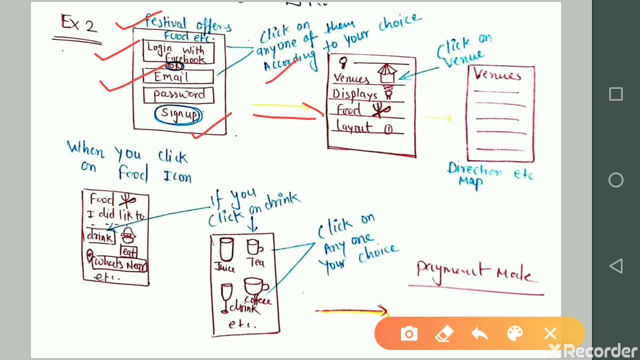 to your choice. we have another window. this is the venue and this is a display: food and layout. these are the options. choose from them so it show you direction. if you click on a venue, this is the direction map. if you click on display, display, all the, all things and food or all items for eating and layout, there are